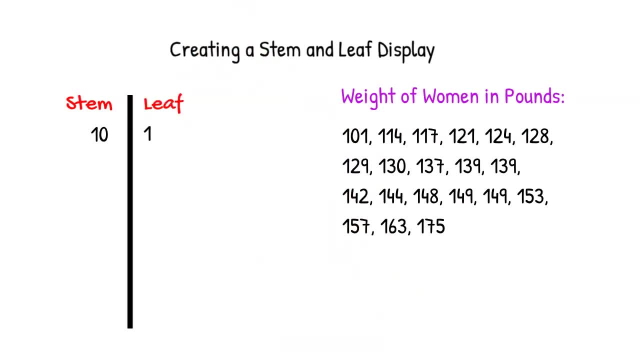 Since it ends in 1,, we put 1 here. Our next stem is 1.. Two numbers start with those digits. The third digits are 4 and 7 respectively. Our next stem is 1, 2.. The numbers in the leaf are 1,, 4,, 8, and 9.. 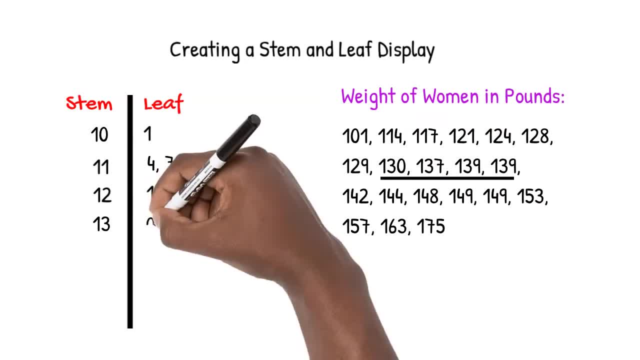 With a stem of 1,- 3,, the values in our leaf are 0,, 7,, 9, and 9.. With a stem of 1,- 4,, the values in our leaf are 2,, 3, and 9.. 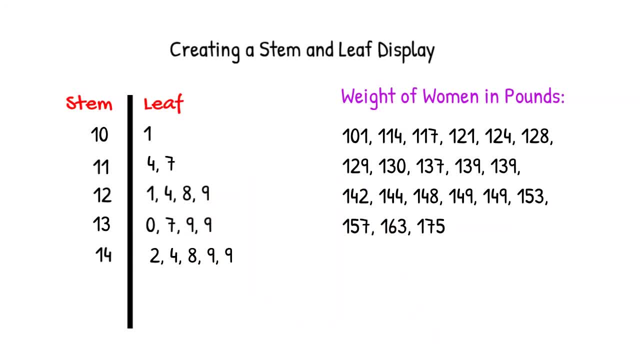 With a stem of 1, 4,, the values in our leaf are 2,, 4,, 8,, 9, and 9.. With a stem of 1, 5,, the values in our leaf are 3,, 7, and 9.. 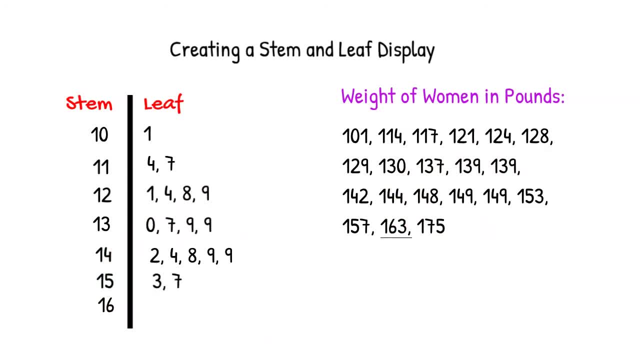 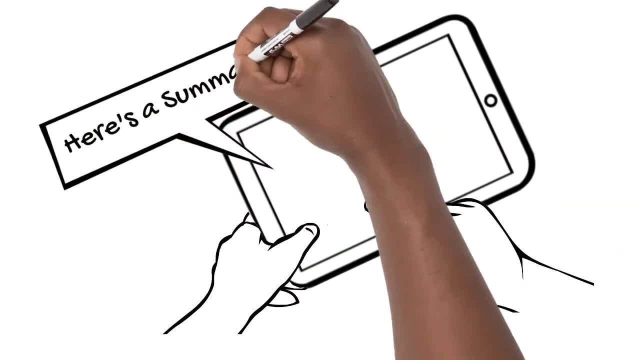 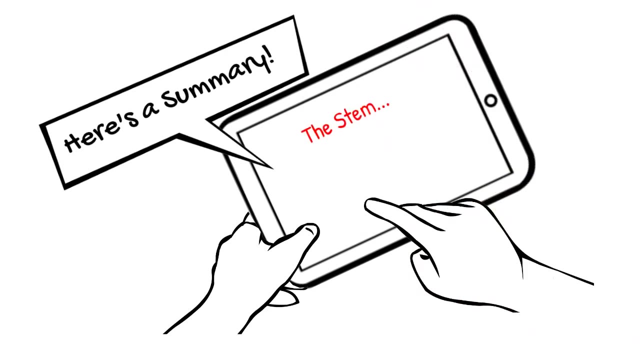 The stem of 1, 6 has 1 leaf 3.. And the stem of 1, 7 has 1 leaf 5.. Here's what we learned in this video. A stem and leaf displays quantitative data. The stem gives the start of the number. 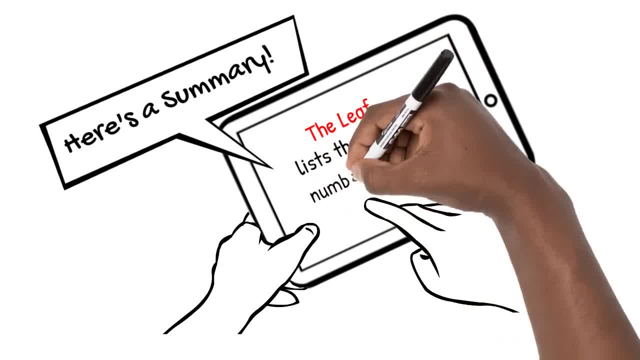 The leaf lists the numbers in each bin. The leaf lists the ends of the numbers in each bin. 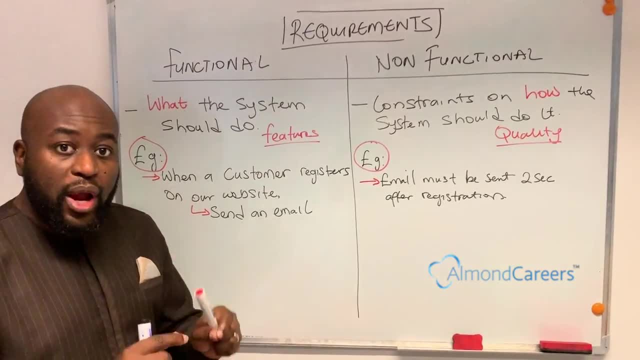 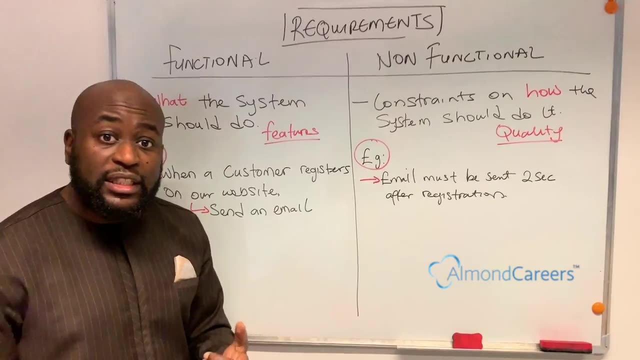 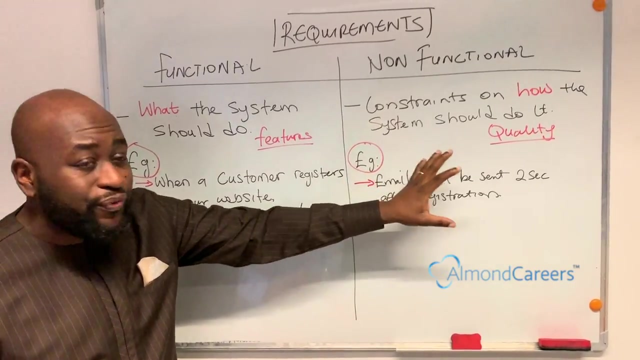 Hi everybody. I'm here to talk to you about requirements, Functional and non-functional requirements. Now, every time most people think of gathering requirements as project managers or business analysts, they are always thinking about functional requirements, But you have to understand that non-functional requirement is one of the most important type of requirements that. 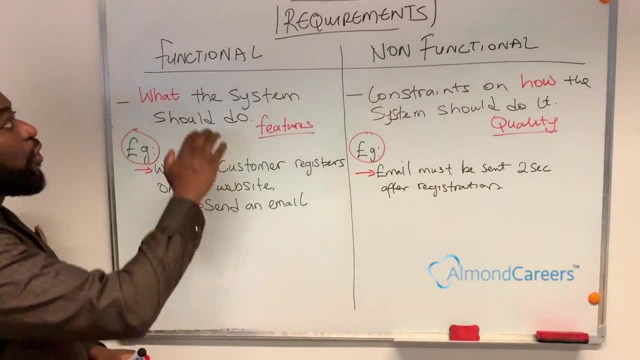 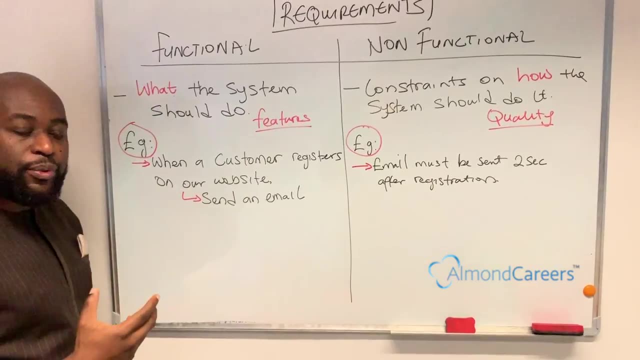 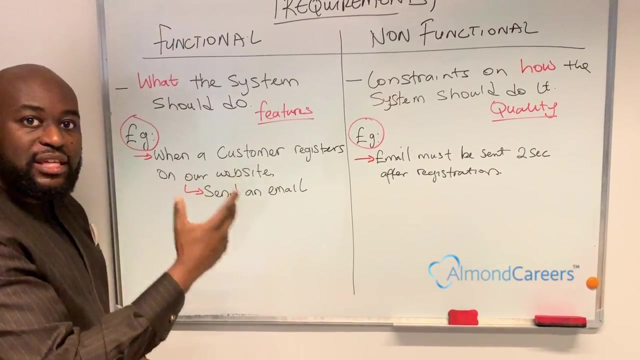 you have to gather as a business analyst. Now, functional requirements describes what the system should do, Whatever it is you are building. the key features, for example, are your functional requirements. I'll give you an example. when the customer registers on our website, they send an email. So you see, that is a.